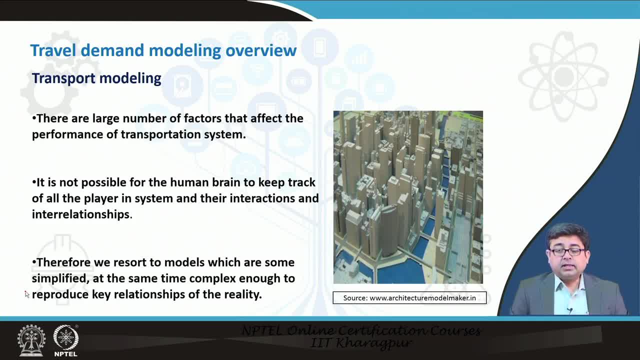 about these modeling techniques, then you can go ahead and take the different in depth courses that are available on this. So when we are looking at transportation modeling, essentially what we are trying to do is we are trying to understand where do people come from and where do people want to go right. 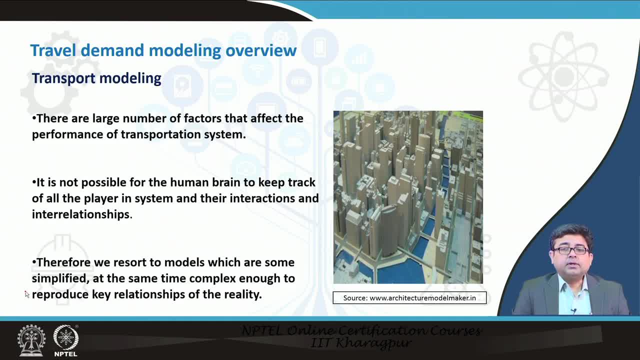 and which route they want to take. So You know where people are staying, where they want to go to, which route they want to take and also what is the vehicle usually they want to go or they want to prefer to use right. do they want to use their own private vehicles, cars or two wheelers, or do they want to go? 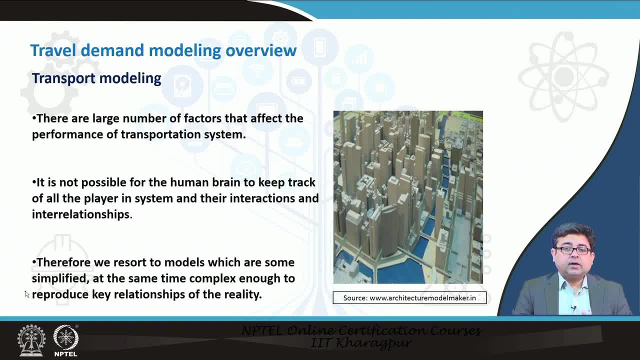 on a bus? do they want to take metro? So if you kind of combine these four aspects of the need to travel, that you would be able to determine At a macro level what is the demand for transportation in your city and based on the demand, you could. 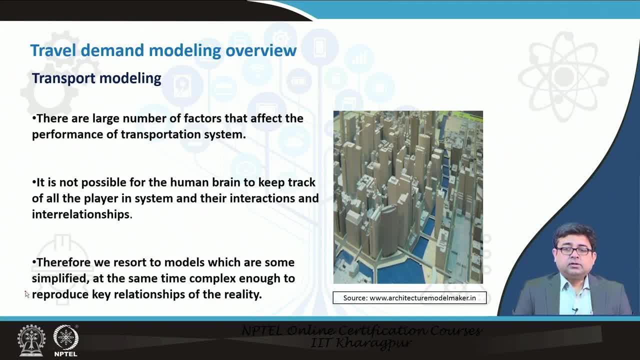 then provide for the capacity, or you can provide for the number of lanes in a road, or the number of bus routes in a in a city, or the frequency of your metro rail, and so on and so forth. So that is essentially what we would want you to. 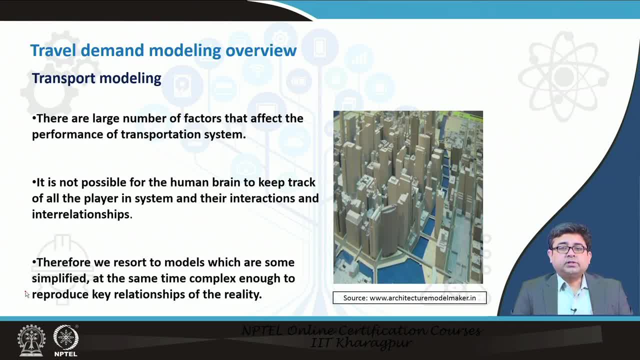 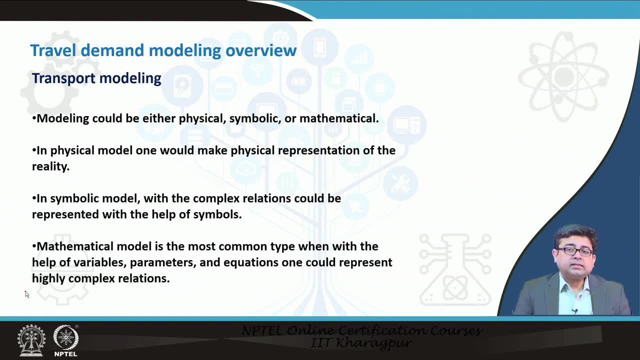 Be aware of when we are talking about Transportation modeling- ah, Number of bus routes in a city, Number of- I mean modeling in general. what a model essentially indicates is that it is a replica of the actual system or the actual network. right, You can build a physical model. right, you can build a miniature car which looks like: 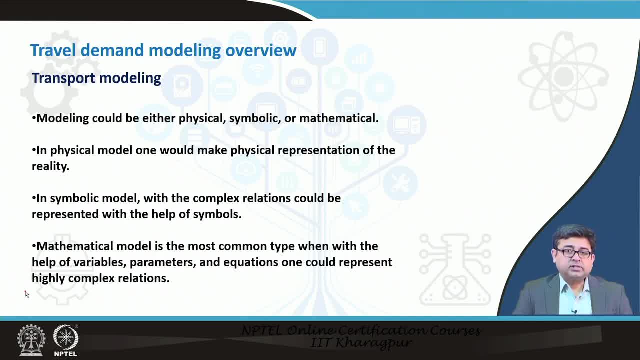 an actual car. you can have a symbolic model which determines a complex system, using different symbols, maybe, or you can have mathematical, statistical models which, by the use of equations and different types of parameters, try to explain how a system works. So when we are talking about transportation modeling, we are essentially talking about 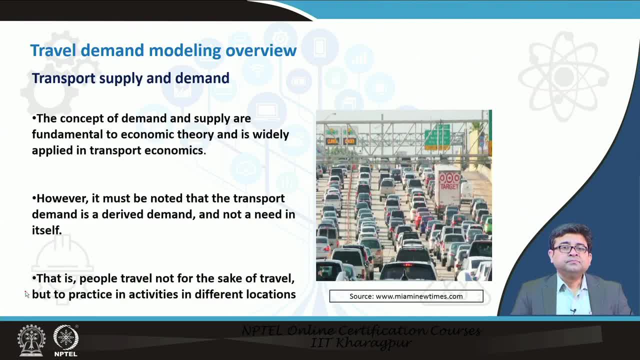 mathematical models. So this concept of travel, supply and demand, so this is essential to the understanding of transportation, This is essential to the understanding of the transportation modeling. So now the supply side of it is the availability of the roads in our city. So that is an example of supply. 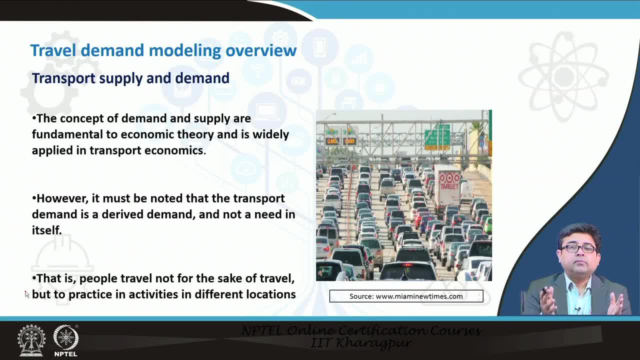 So I have n kilometers of road in my city. So that is the supply of the transportation network. Another example would be: I have 49 bus routes in our in my city. Each of those bus routes have a bus frequency of one bus in every 10 minutes. 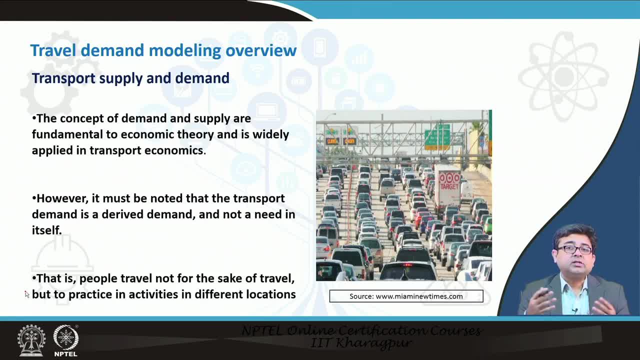 So that tells me that you know the capacity of the bus right and you know that every bus comes in every 10, one bus comes in every 10 minutes and you have 49 such routes, then you are, you know the capacity that the buses bus network can carry. 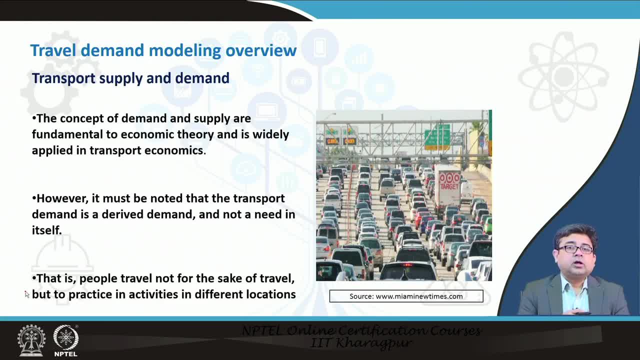 So that is like the supply side. Now, when you talk about the demand side of things, then you say that, okay, now you have, for example, n kilometers of highway, but how many actual vehicles are there in your city that will use these highways right and for how much time will they use it right? how much? 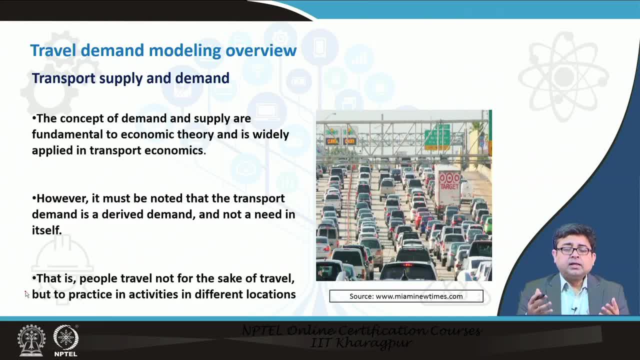 time, or how much, how many kilometers will they drive? So you have to know both. you have to. it is easy to know the supply side because it is actually either Existing or you, it is planned. So you know that. well, in the next five years I am going to build n number of n kilometers. 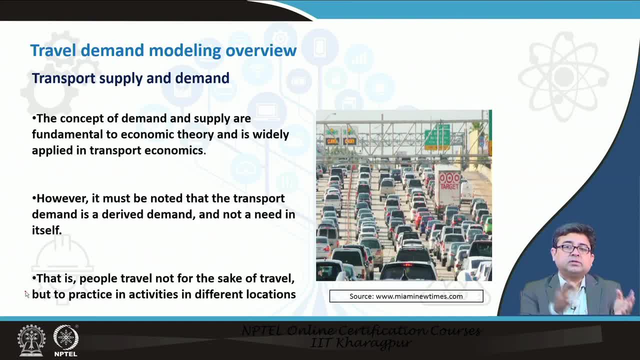 of roads or I am going to have n number of buses, new buses in my fleet, But when it comes to demand, you are you. you almost cannot absolutely know what the demand is right. There may be new vehicles, people coming into the city buying new vehicles. 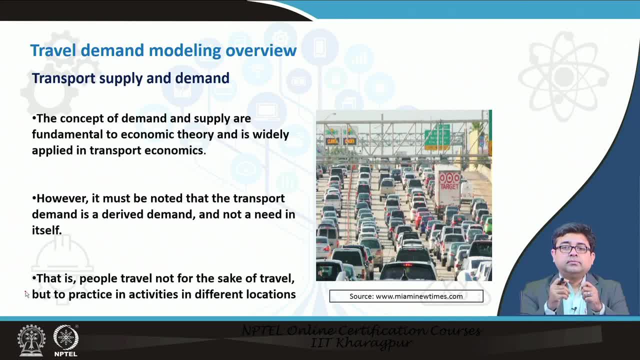 So you do not. you actually cannot accurately predict, Okay, Or you cannot accurately count the demand. So what you essentially end up doing is you end up estimating the demand. So when you are trying to end estimate a demand, that is where all the models or the demand 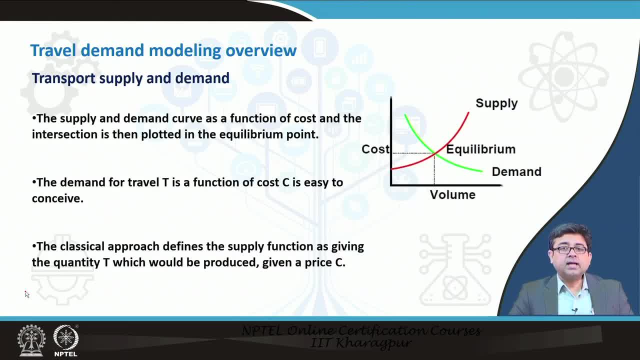 models come into play. So when you look at the supply and demand curve, it is a classic economic example of for anything, for any entity. When you look at the cost versus volume, Okay, You say that if, if, the number of, if the supply of certain things, 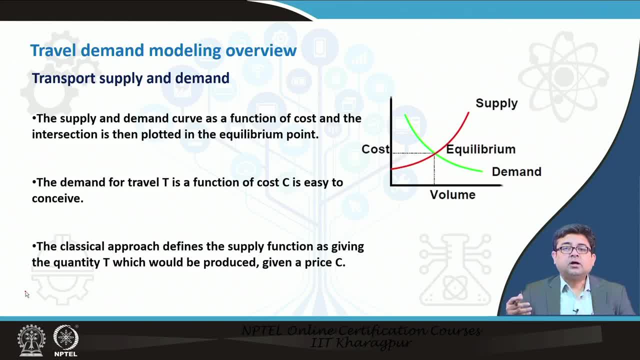 So the volume of certain things increase, the cost of it also starts increasing, right? So, if, if something is selling very well, right, if, if, if, if cost is very, if, suddenly, for example, a, a, a, a person manufacturing soap, start seeing that the soaps are selling very well. 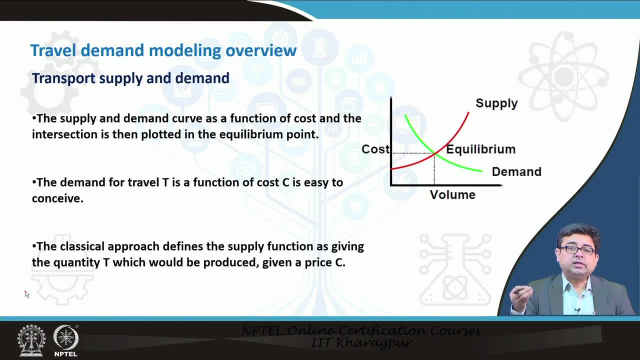 So he increases the manufacturing or he increases the volume of the soaps manufactured and also more and more people get into the soap manufacturing business. So the the the cost that he gets out of selling these soaps, keeps on increasing, So the supply keeps on increasing. the supply is always the upward, moving, upward sloping. 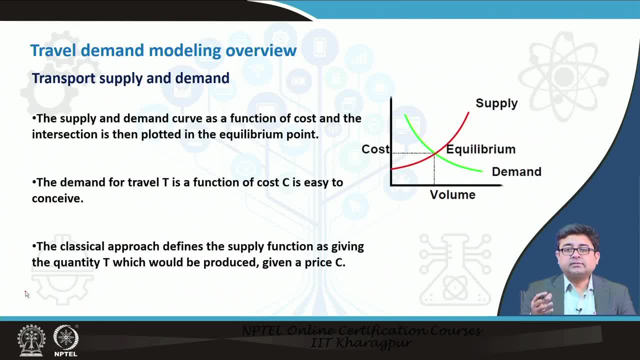 curve, whereas demand, so as as, as as the volume of goods starts increasing from the demand side. So people who want to use the soaps, the cost for them starts decreasing, right. So competition brings down the cost for them. So that is the always a downward sloping. 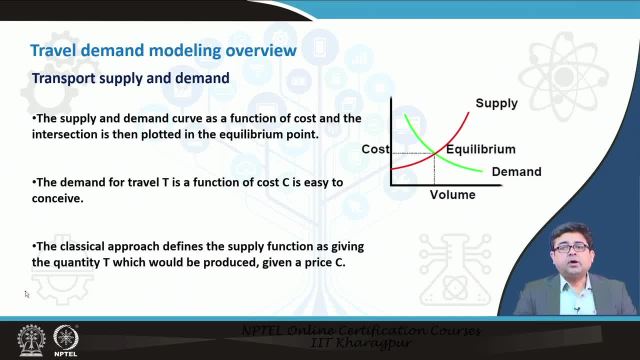 So, similarly, when you are looking supply and demand from the point of view of transportation, you say that when, when you provide, when you provide for multiple transportation systems in your city, usually the cost of traveling goes down. Okay, When you provide for one type of transportation, for example, private transportation, private. 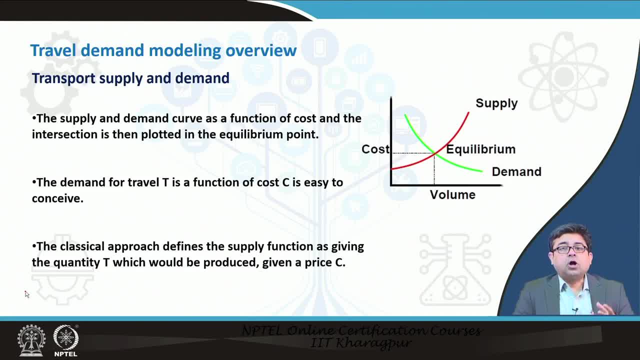 motorized transportation. So then what happens is the cost for travel always remains high or keeps on increasing. So always the demand decreases as competition, or the or the price per price for entity decreases as competition increases. So you are always encouraged to have multimodal transportation network. 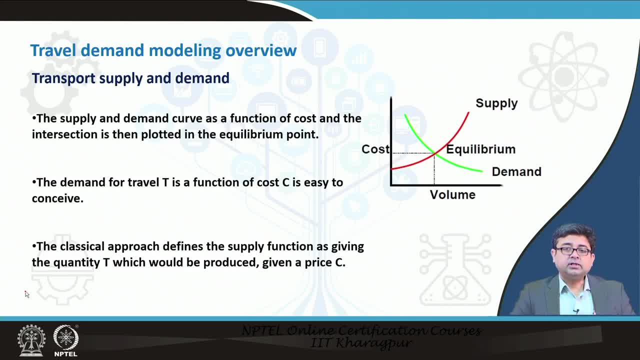 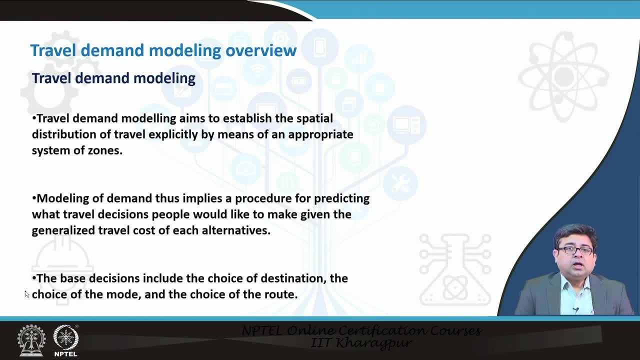 In your, in your city, which will eventually bring down the costs for your users. So when you look at the transportation demand modeling, it aims to establish the spatial distribution of travel explicitly by means of appropriate system of zones. So what? usually we will look at it in the in the next slide, in a step by step manner. but 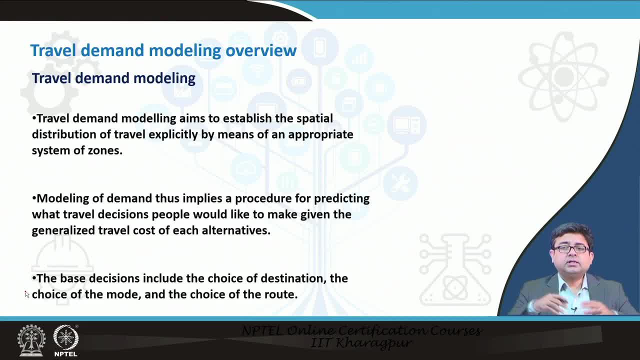 what We are saying is that your, your city, could be vast right. So to exactly know where people are traveling to and from maybe very difficult. but on a macro level, on a on overall level, you can. you can say that people usually in the morning would travel from where they live to where they work. So if you know the land uses residential. 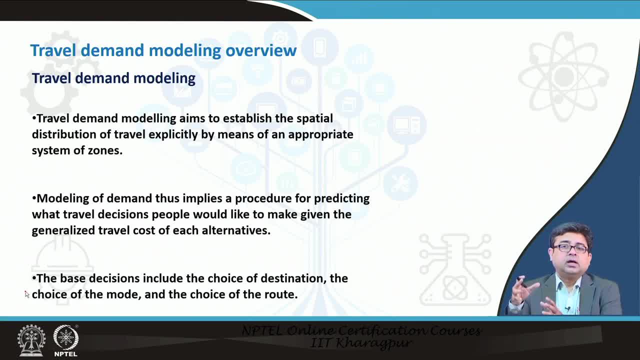 predominantly residential land uses and the predominantly commercial or office land uses. So you would know, or you could predict with certain degree of accuracy, that the traffic will flow in a direction which is from the residences to the office buildings and similarly, in the evening it will be the opposite traffic flow. 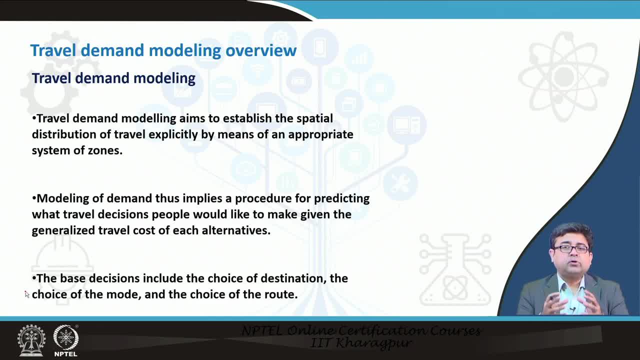 So that is kind of at a macro level. your prediction is accurate. However, it becomes very difficult to predict it during the middle of the day and also during the weekends. It is weekends: people take a lot of leisure trips. in the middle of the day, the trips. 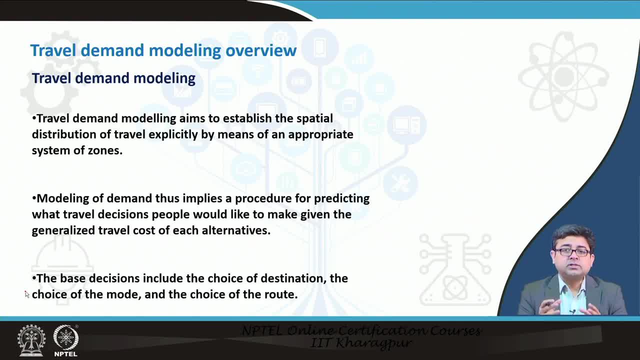 are usually taken by non-commuters. So when non-commuters, meaning non-office goers, make their trips, then you really have difficulty in predicting where they are going and you need very hard, So you need very high data about the land uses and the trip purposes to predict exactly. 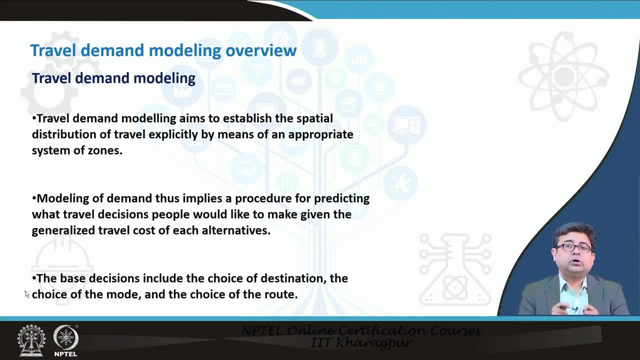 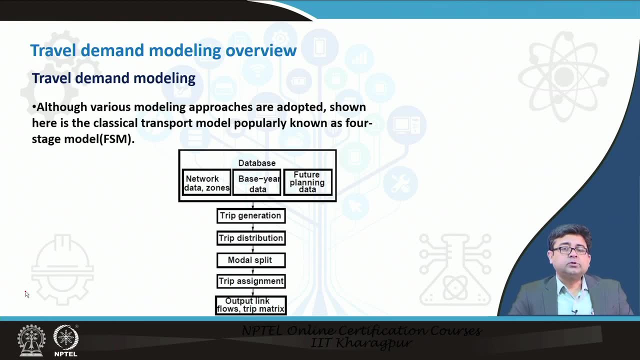 where people are going, so that you ensure that you provide adequate capacity of your transportation systems to meet the needs of the travelling people. So in here, what we will give you a brief overview of is the most popular four step model of mobile demand estimation right. 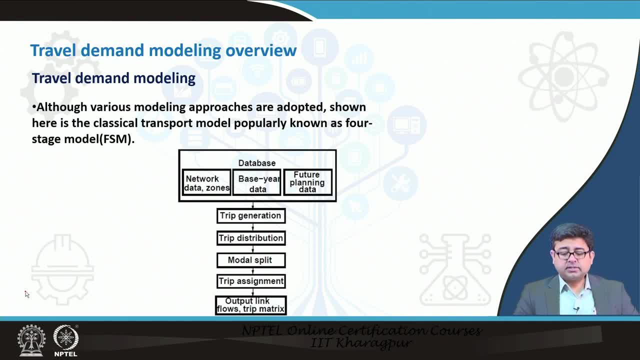 This is a popularly called the four stage model, and the first stage in this is what is called trip generation. the second step is trip distribution. third step is understanding the modal split, or the choice of mode that you want to take. and finally, what is the transportation? 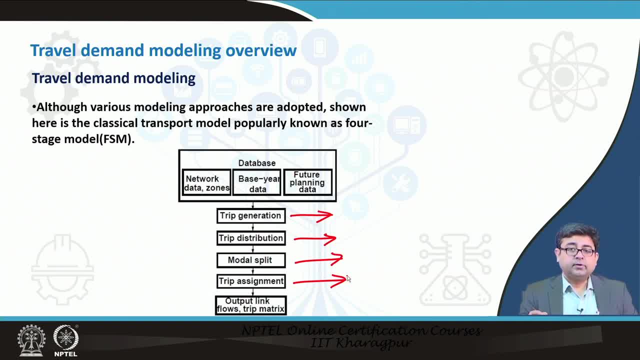 network that you will be using when you are going from your office. You will be using the Ed hj offerings or the the July options option. Basically, how could you do that? So if you go to these four, have to have certain amount of data, ah that feeds into, ah the acts as input or feeds into. 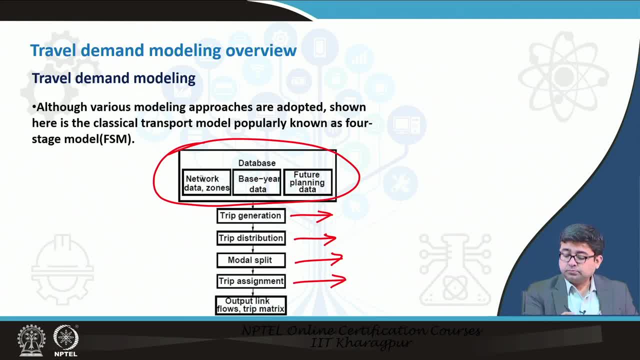 your model. So you have to know ah what is the existing network that you are working on ah you have to know how many vehicles currently ah run on your ah network. and you also have to know ah some future planning ah based on the ah comprehensive plans that are available- comprehensive. 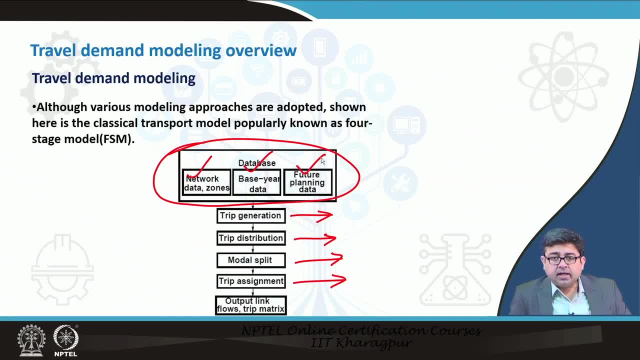 mobility plans that are available for your city or the city's master plan, which must have ah incorporated, a 20, 30 year horizon plan ah, which must have incorporated how many roads there will be, how many kilometers of roads there will be 20 years down the line. 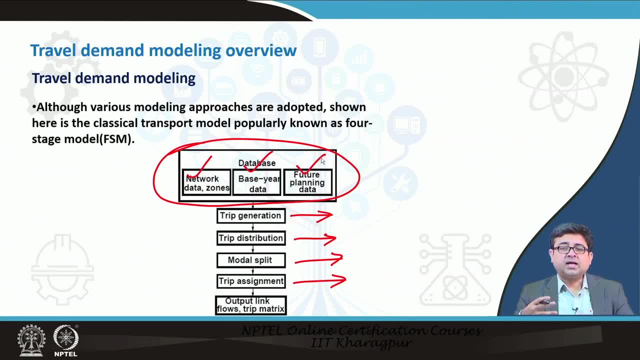 So all of that information has to be fed into this model as an input, and then this model would be able to predict that how many trips or how many vehicles will be on the road in a next year, five years down the line, and so on and so forth. So the model starts: ah, if I, if I were to give. 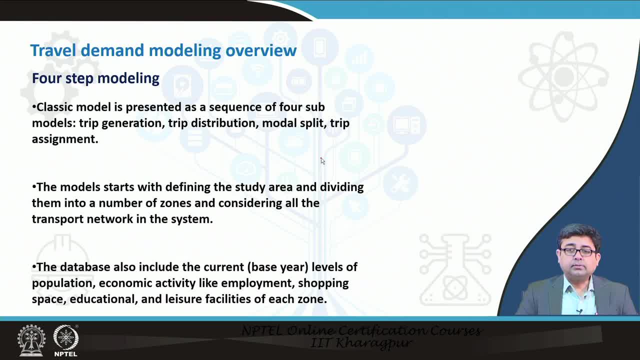 you a basic example, ah, or a very ah, ah, ah, ah. explanation of this in a nutshell: ah, the first, ah, the first step in this is is is trip generation, and for trip generation, usually what you do, What you develop is, ah, ah, a small zone of your city. 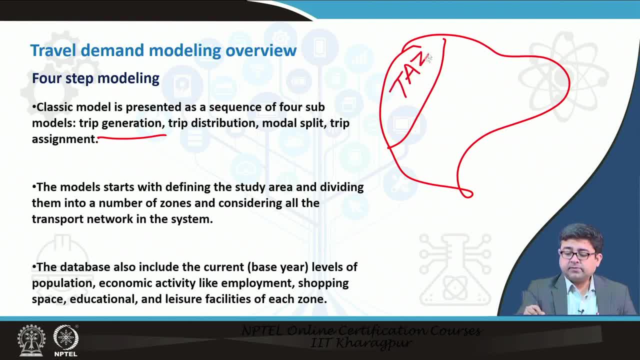 ah, which are usually called TAZs- traffic analysis zones. So you divide the entire city into different types of traffic analysis zones and this is called a macro model, because now it is going to use this zone, ah, at a macro level, to predict how many trips. 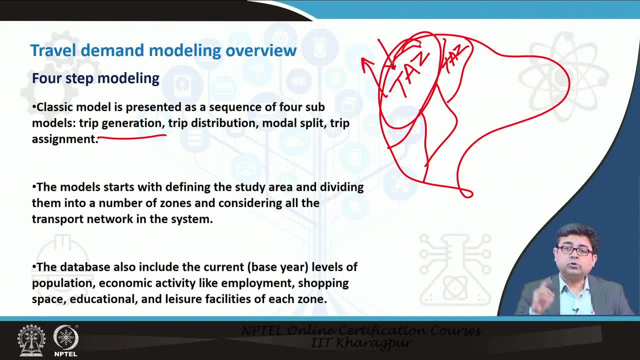 ah and exiting this zone. So remember, we are not doing it at a micro level, So we are not tracking everybody's ah movement to realize or to predict how many trips are going to be coming out of ah, your ah or coming on to the network, but we are doing it at a macro. 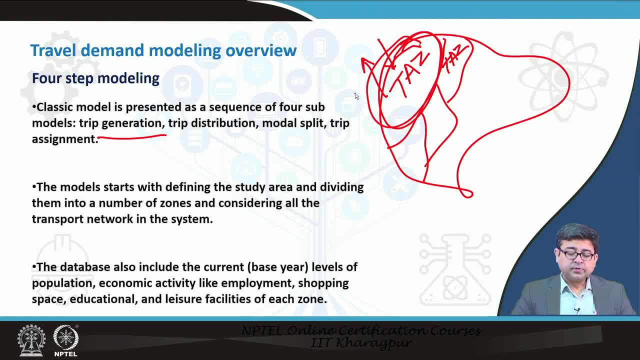 level, at a level of a traffic analysis zone. So we divide, first of all, we divide it into all of these zones, ah, and then we look for all the socio-economic data, ah, for the families that are living within that zone itself. right, that acts as an input. We are look, then we. 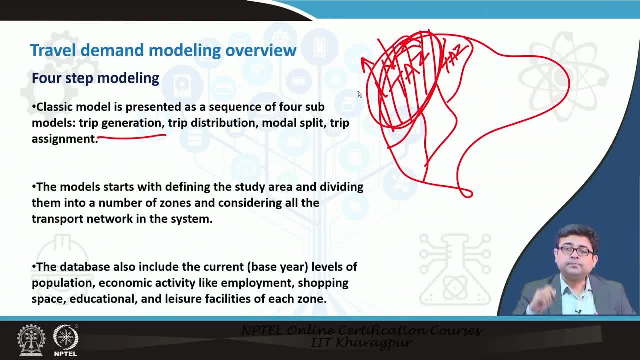 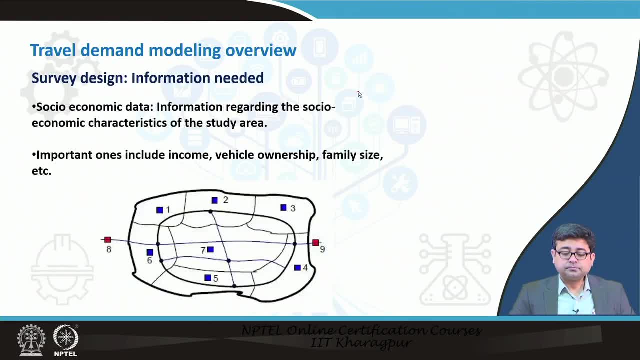 look at all the highway network or the roadway network within that zone. ah. we look at the socio-economic data and so on and so forth, So that it can be fed into the model. ah. several types of surveys need to be conducted ah in order to get all this information. 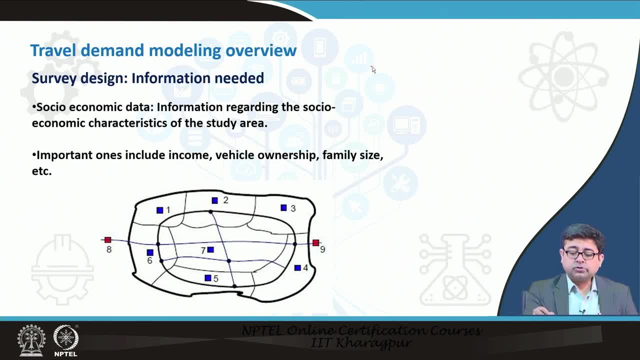 ah, You have to, ah you have to conduct household surveys, right. So ah household surveys are very household travel surveys are very similar to ah your census surveys ah that are done, ah census surveys that are done, where ah surveyor would ah come to your household and ah ask. 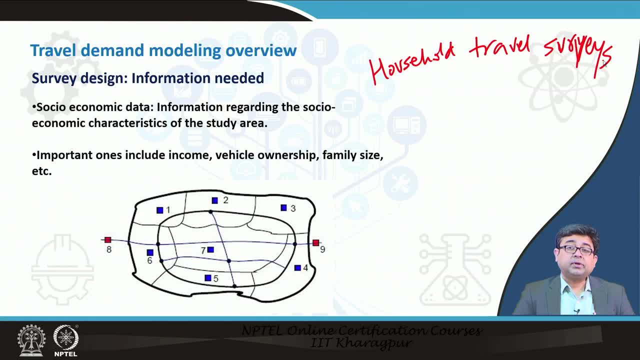 you a certain number of questions ah about ah typical trips ah that you take ah during a weekday or a weekend ah. So these obviously are anonymized ah there is no information about. there is no ah ah data about who you are or what your ah ah what your ah identification is. we ah the data. 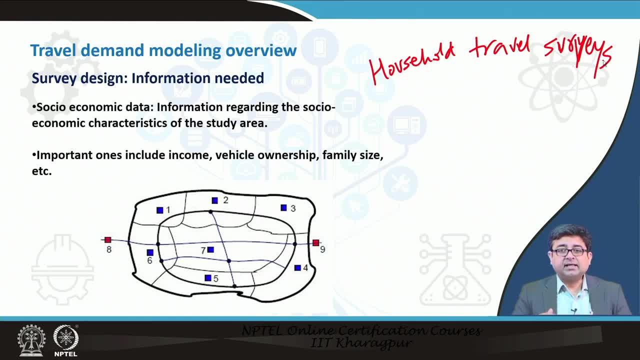 is ah just required for ah different categories of households, So households by income, households by age group, households by ah- number of cars you own. So the data is categorized in that manner rather than ah with any of your personal information, ah. so that is. that is one type of survey that 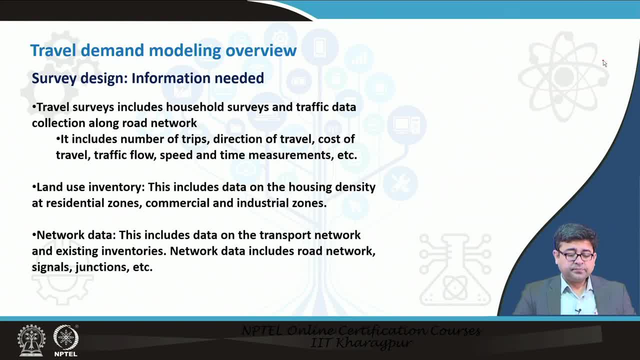 is conducted ah. the other type of surveys that are conducted ah include, ah traffic data collection along roadway networks. so, ah, you would have to have an information about what is the existing volume of traffic on your, on your, highways. So in order to do that, ah, you have to ah, ah collect data. 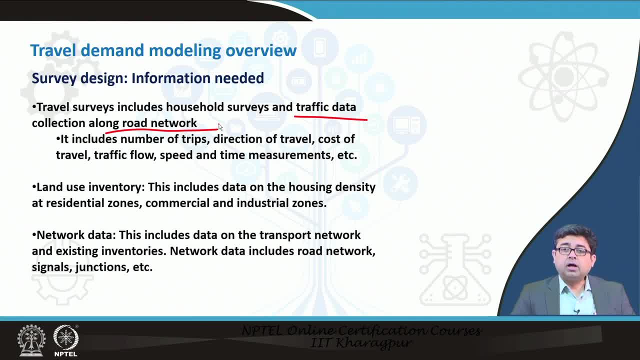 about the traffic volume on your roadway network. nowadays, like i had mentioned earlier, you have cameras throughout your transportation systems, which makes it easier to at least gather this data. so once you have gathered, collected this data, you have to analyze it, you have to clean the data and and and convert it into information which will let you know that the number of trips that 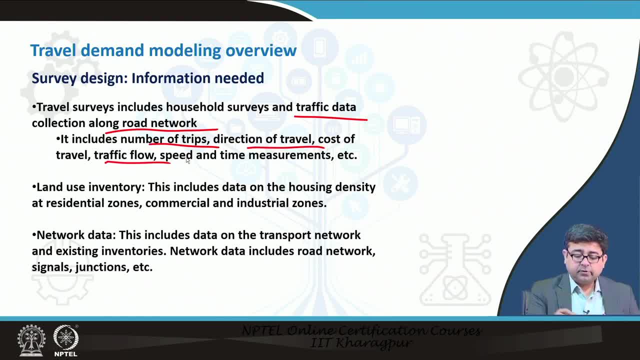 are being taken, the direction of travel, the traffic flow and the speed, so all of these estimates can be made. once you acquire or collect this kind of data, along with it you have to understand, you have to have data on your land use inventory which can be collected from urban, local 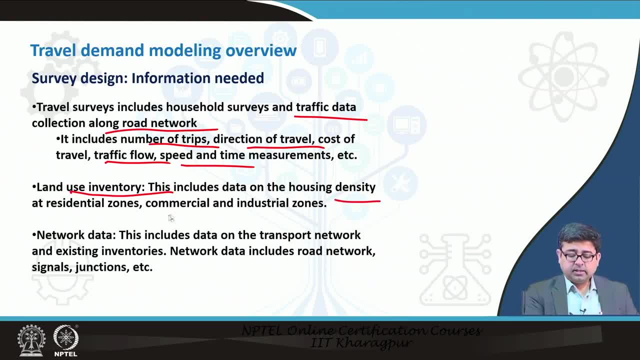 bodies, the housing density in commercial, residential industrial zones. that has to be also collected. and, of course, you have to know your base skeleton, base skeleton, uh. the network data about your highway, about your roads and highways in the tag. so let us always remember that we are all collecting this at a traffic analysis zone level. 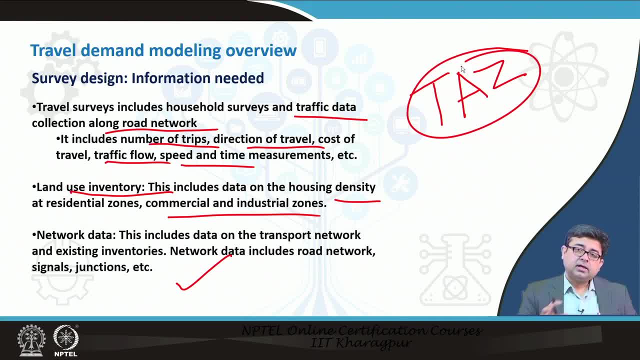 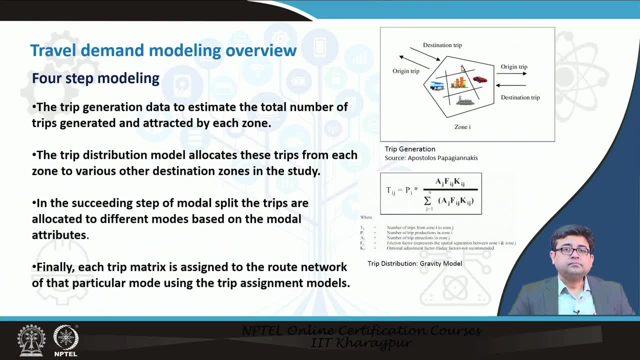 so once you divide it up, divide your city into different analysis zones, for each of these zones, you will have to have these kind of information. now, what the four step model does in the first step is that it estimates how many trips are being generated from each of those tag's right. so so this is a zone. 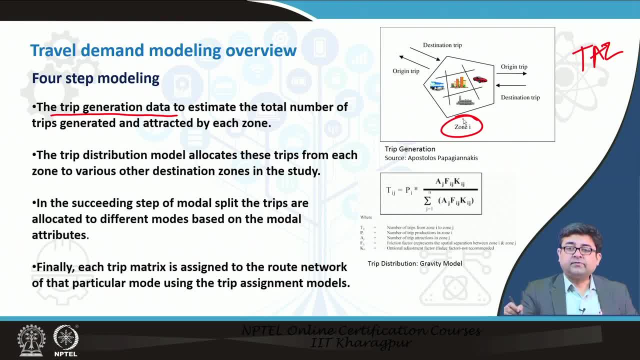 one meaning or zone. i meaning that is one of the traffic analysis zones. so it what it essentially does is just counts the number of trips that are coming in and the number of trips that are going out. so in other ways you can say that these are production trips that are going out and these are 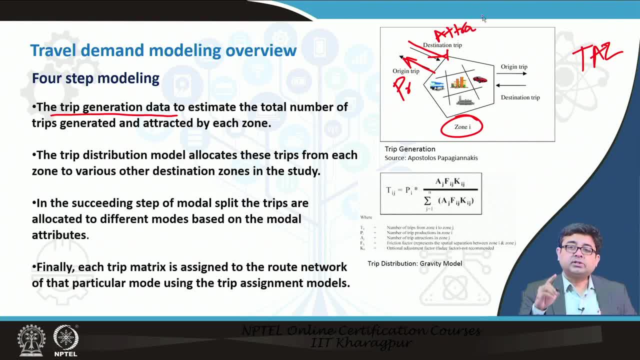 attraction trips that are coming in. so trip is just a one, one way travel between point a to point b. it is, it is not a round. ah, it is not a round trip, it is just a one way trip, so any. so this is one trip and this is the other trip and if any trip is being produced is an outward. 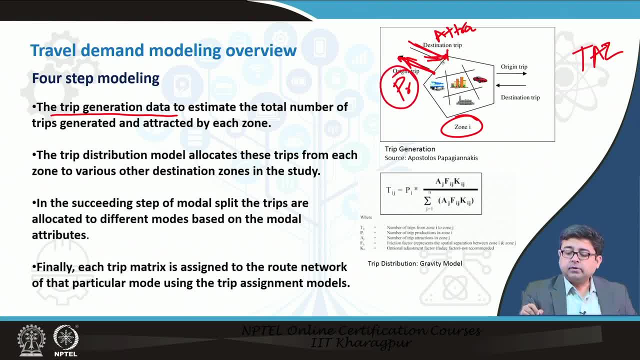 trip, it is called a production trip, whereas anything that is an inward trip, the zone, is called an attraction trip. so the first step in the four step model only does that. it it develops an estimate or for the number of trips that are generated, or, meaning, produced and attracted by 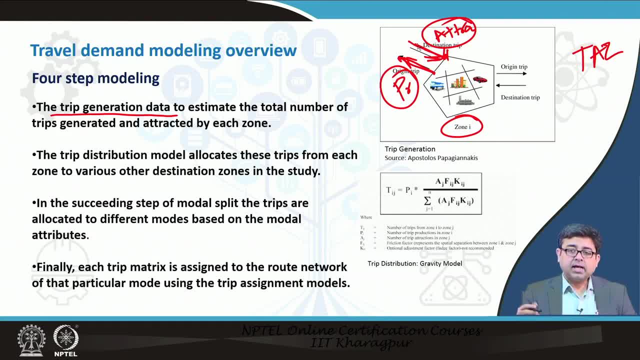 any particular zone, then, once you know that, the second step or the trip distribution step it. what it says is that now that this trip, now that we know how many trips are being generated, we have to assign those trips to other zones right now if the if the trip is being produced. 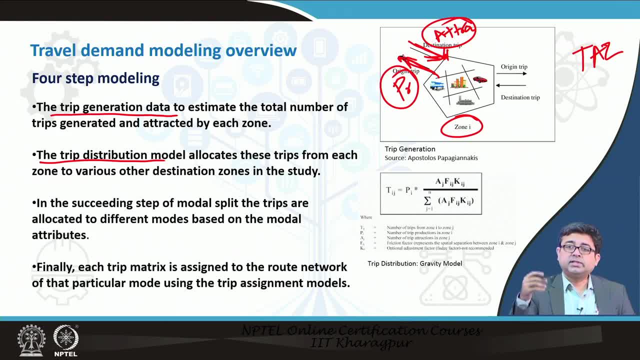 from this zone it must be going to another zone, so which is that zone, right? so we need to assign it to that zone. similarly, if a trip is being attracted to this zone, it must have been produced in some other zone. so where is this trip coming from? so the trip distribution. 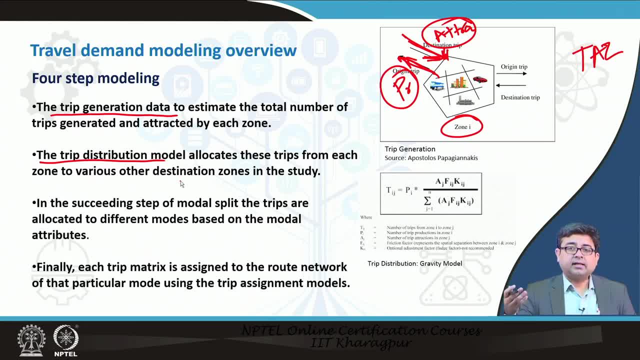 model kind of predicts that it predicts where these trips that have been generated are coming from or going to. so usually the most common model that it develops is the gravity model. so it says that trips between two zones are directly dependent upon the attractions that are available in the in the other zone and the distance or 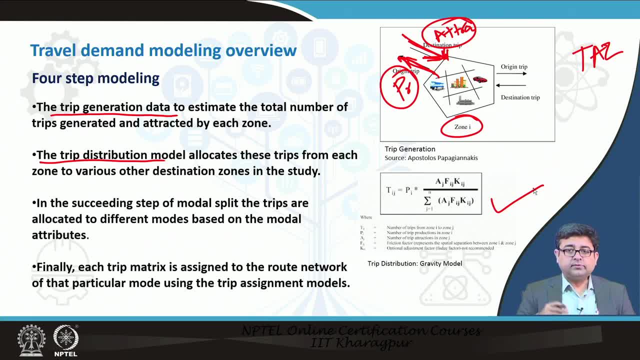 travel time or one of the other, between those two. so if there are lot of attractions in a zone, then it is likely that a trip that is produced in one zone is being attracted to that zone. so attractions meaning an attraction could be a movie theater, a park, a restaurant or 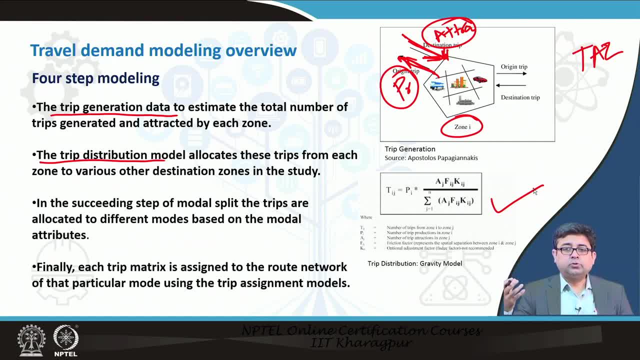 number of restaurants. so usually, if you want to say that, residential zones are usually production zones in the morning and office areas are normally the attraction zones in the morning, and whereas in the evening they reverse back, and so the office zones become the production zones and the home zones become the, or the residential zones become the attraction zones. 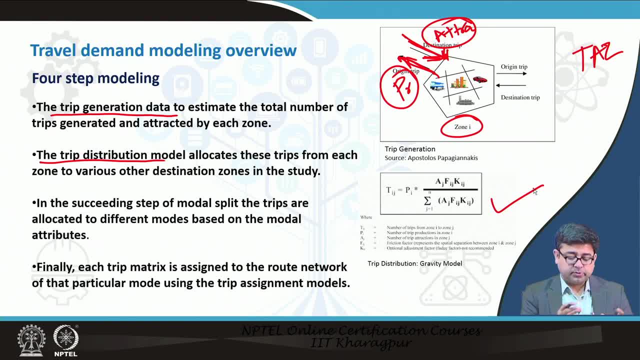 so that is what the trip generation or the trip distribution model does. in the next step, once you know where these trips are going to, between which zones are the majority of the trips going, it is essential, it is essential to understand how they are going there. so are they going using two wheelers? using four wheelers? using metro rail? are they walking? 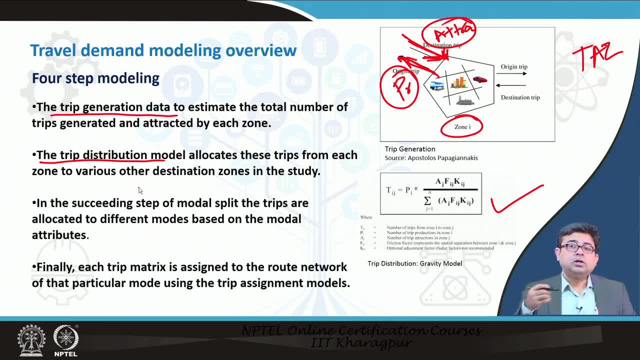 to these zones? are they using the bicycle? so what is the choice of mode that they are taking up in order to travel from this zone to that zone? so that is, that is, that is a step called modal split and finally, once you know the zones that they are going to, and 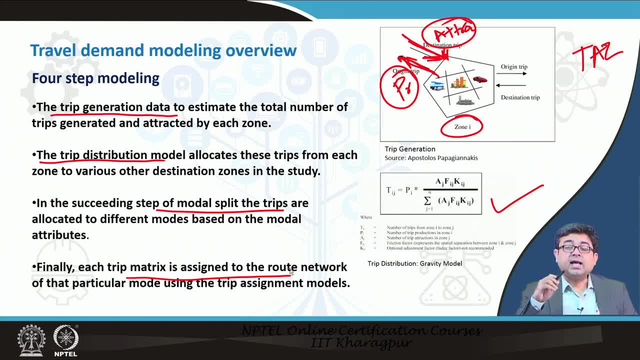 the road that they are using. you can assign that trip to the network that you already have, so you can say that, okay, from to go from a to b there is no direct metro route, so it is likely that this person will take his or her private vehicle and this is the road, or? 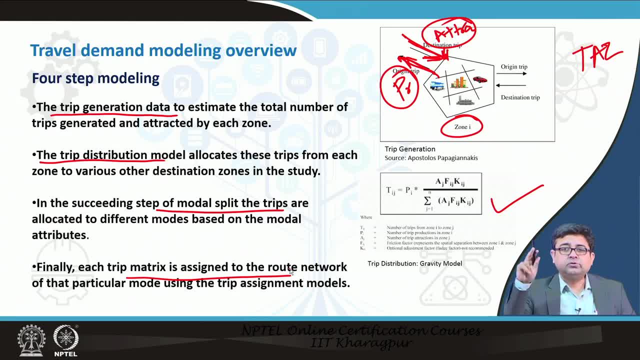 the shortest road, shortest travel time road between these two zones, so let me assign this trip to that zone. So essentially now you will know that a particular trip that was generated in one zone is being attracted by another zone or is distributed to that zone and is using personal.